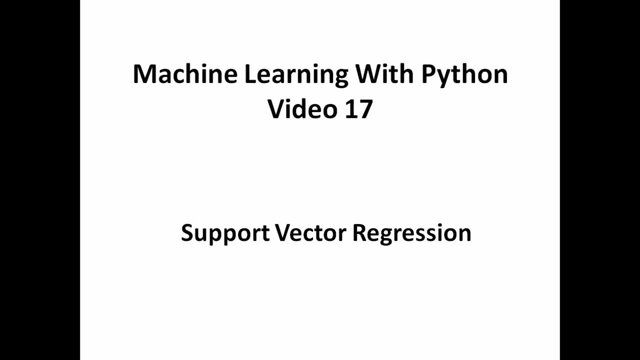 Hello Python Programmers. so this is the video 17th of a Machine Learning with Python video series, and in this video we are gonna discuss about Support Vector Regression. So, just like our previous videos, this video is also divided into two sections. In first part we will see: 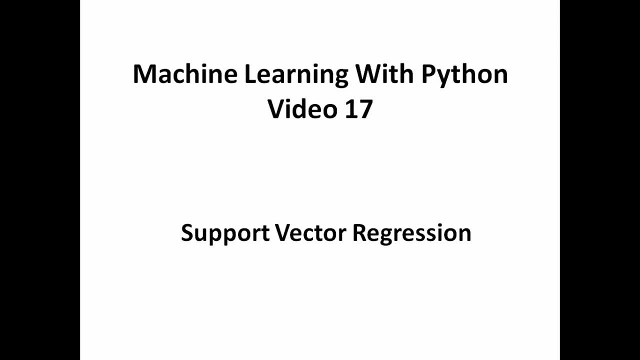 the theoretical explanation of what Support Vector Regression is. that is, what is happening in the background of Support Vector Regression. Then in the second part we will work on actual data set and see practically that how Support Vector Regression works. So first let's see our first part. that is the theoretical explanation. So Support Vector Regression is a part of 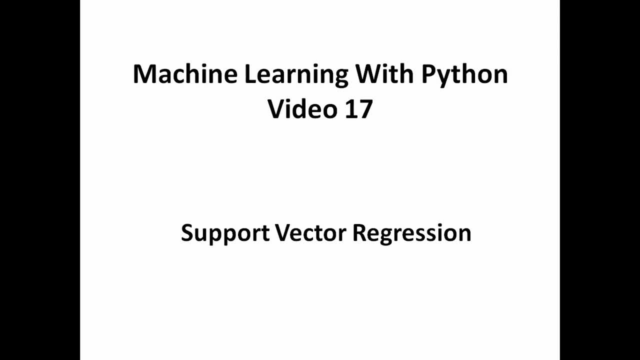 Support Vector Machines. Now let me explain this more clearly. Let's say that there exists a concept called Support Vector Machine, And that concept can be applied for both regression as well as classification data. Now, if you don't know that, what is regression and classification data? I will provide the link in the description. 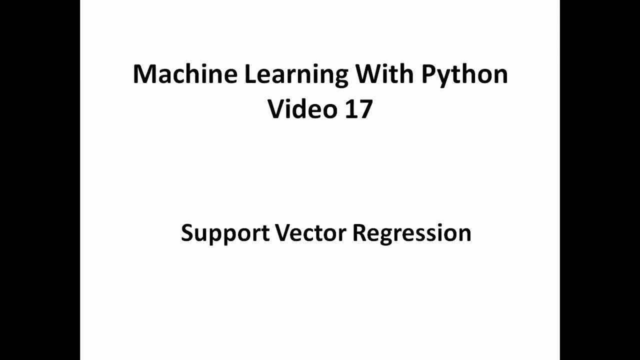 as well as in the i button, so that you can understand that what is the classification of machine learning models? So when the Support Vector Machine is applied for classification, then it's called Support Vector Classification, And when this concept is applied for regression, then that model is called Support Vector Regression. 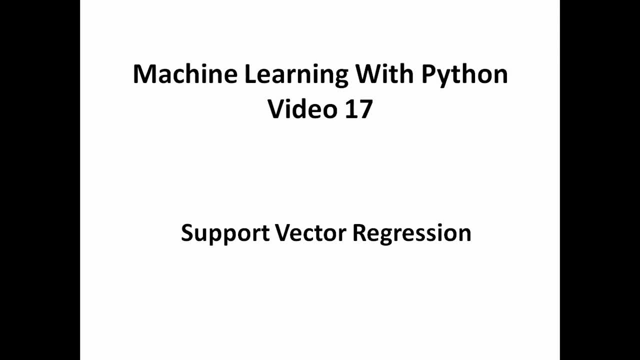 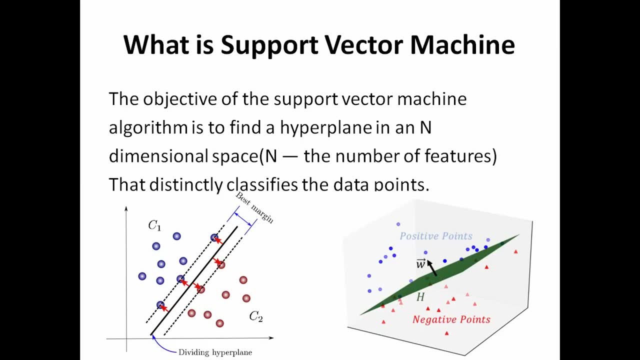 So to understand Support Vector Regression, you must understand Support Vector Machines. So let's see what is Support Vector Machine. The objective of Support Vector Machine algorithm is to find a hyperplane in a n-dimensional space, Where n stands for the number of features or the number of independent variables. 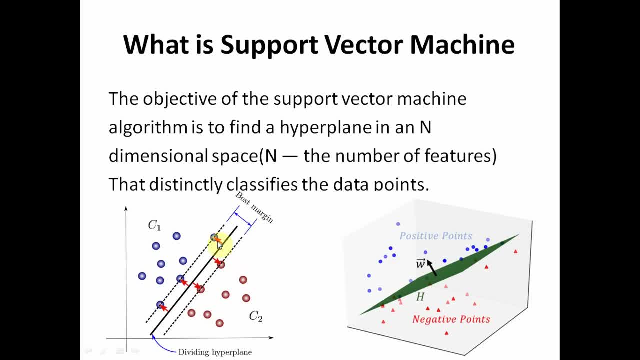 So let me try to explain you with an example. Let's say that this is the tail height and tail width of, let's say, dogs and cats. We are taking the example of classification, but this is just for the explaining of Support Vector Machine, because in majority of cases, 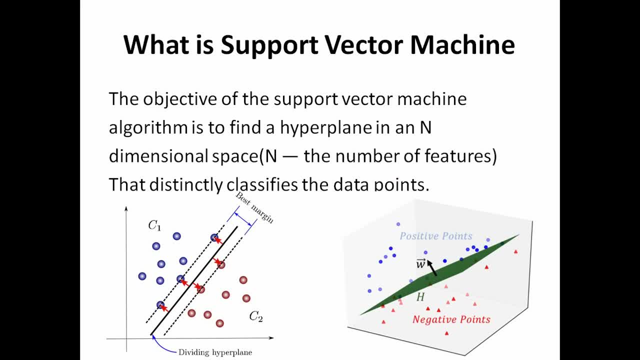 Support Vector Machine is used for classification, And this concept works brilliantly for our linear data. So let me first explain you what is Support Vector Machine. Lets say that the X-axis denotes your tail width and the Y-axis is your tail height. So this C1 part, or these blue data, 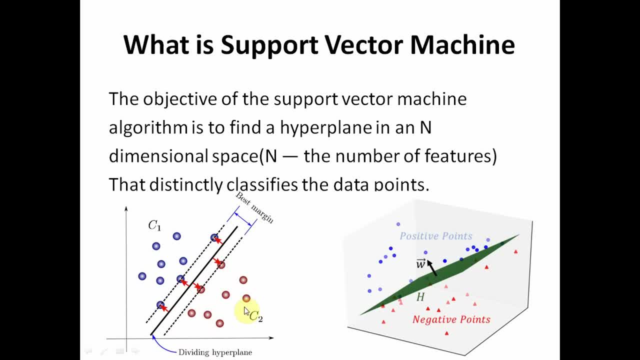 points represents dogs and this C2 represents cats, So there are some data points which are going out of their league there. you can see these are the marginal data points. let's say that there is a dog which resembles very much to a cat- actually its tail resembles very much to cat- so that data point will reside at the 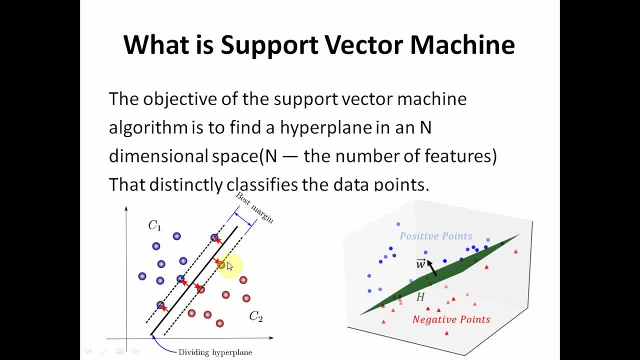 very corner of your graph, and the same happens for the cat. so what we do is we take our extreme points and try to draw a hyperplane between them. so this dark black line is your hyperplane, which divides your extreme points with the equal distance. okay, so this is the best fitting margin. 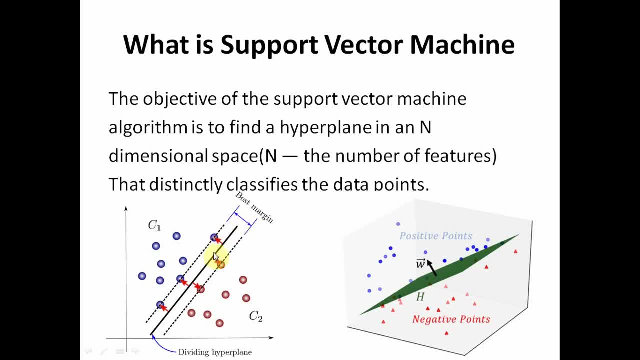 the best fitting margin is the distance between your hyperplane and your extreme points. these are your extreme points. i'll just explain them. okay. so this is the same representation in 3d. if the data is somewhat mixed, then you can use the 3d representation. 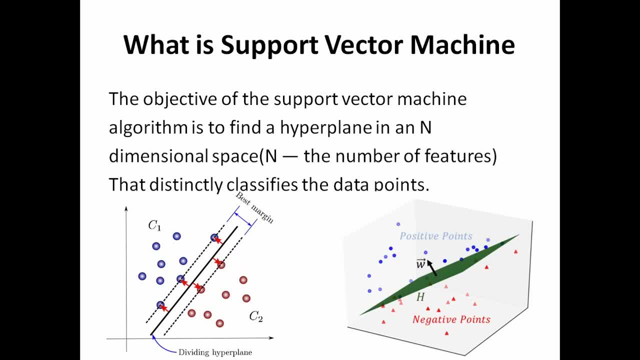 okay, so this is what support vector machine was. we were using hyperplane and best fitting margin to differentiate our data. now this concept can also be used for our linear data. let's say that our data is plotted in a linear pattern. then we can use hyperplane to draw the line for them. okay, so this was the theoretical explanation. 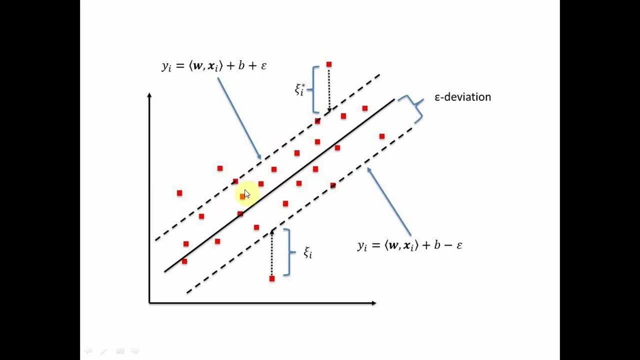 now this is a example explaining you how this support vector machine can be used for our linear regression data. there you can see, this is the hyperplane plotted at the equal distances from the extreme ends. and there you can see, this is the best fitting margin and we can. 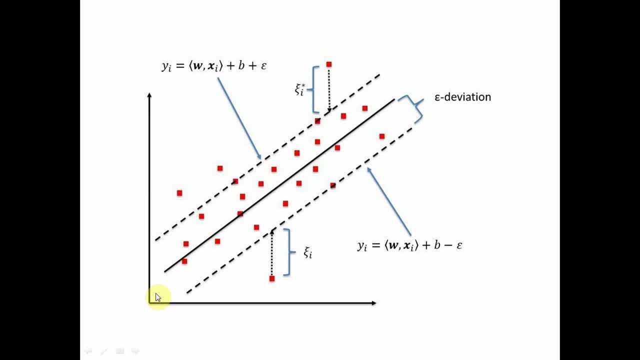 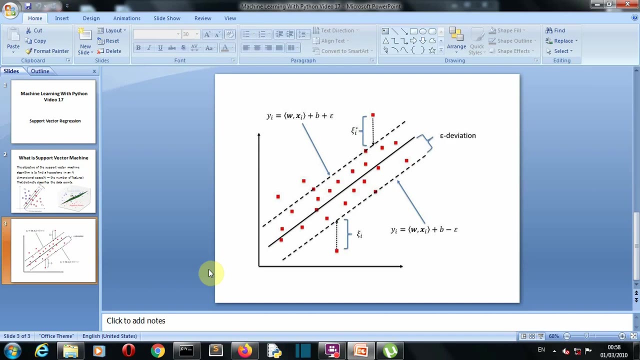 use this method to get our prediction okay. so this was the theoretical explanation. i'm not pressing too much in the theoretical because this isn't used that much for regression. we'll discuss this more deeply when we come to our classification, because this is mostly used for classification. okay, 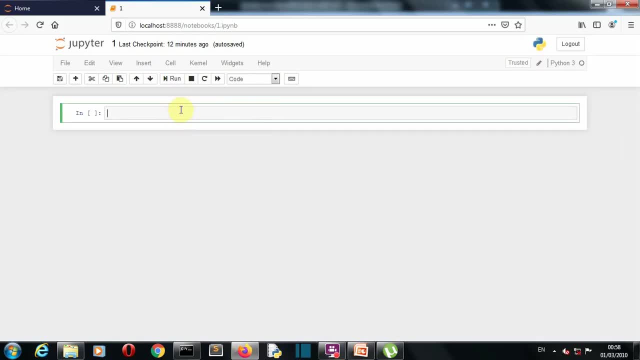 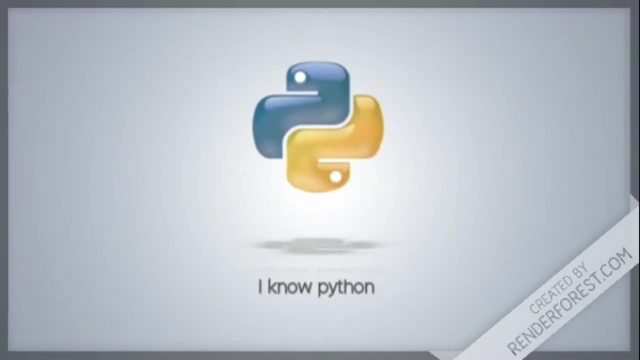 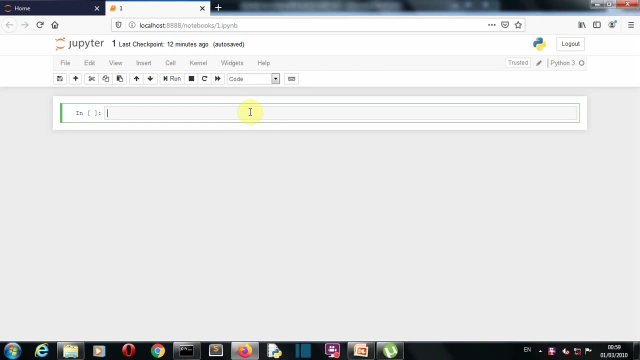 so let's go to our notebook and start writing our code for this. ok, so now our first task is to import our required libraries, that is, pandas, numpy and matplotlib. ok, so there we go. now let's import our dataset. so we'll be working on the detailed. 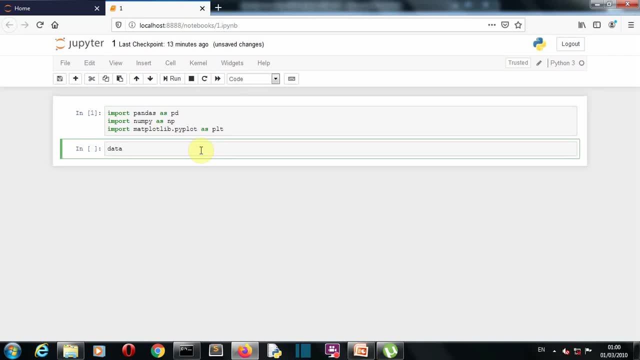 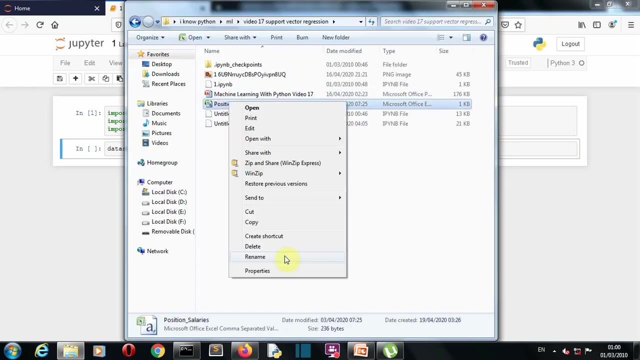 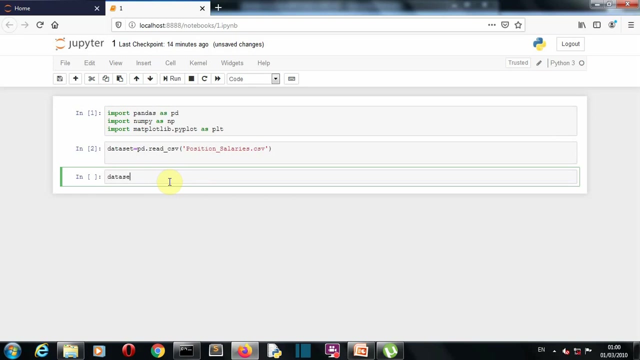 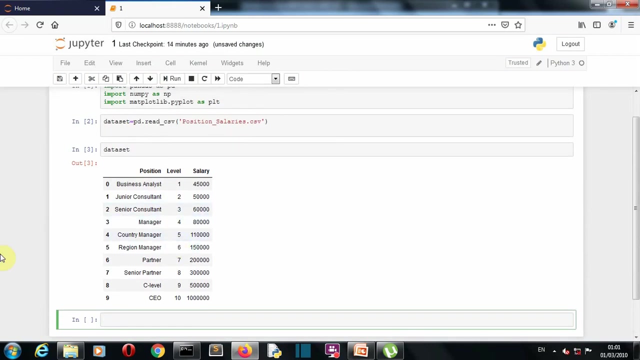 layout in the future using param出来 Puja桑, aunya. so we are going to jeito din ka, st Mentı, st mahi. we definitely need this map, the same data set that is our salary position. so let me import that now. let's see how our data set is looking. there we go. this is a very small data set, if you want to. 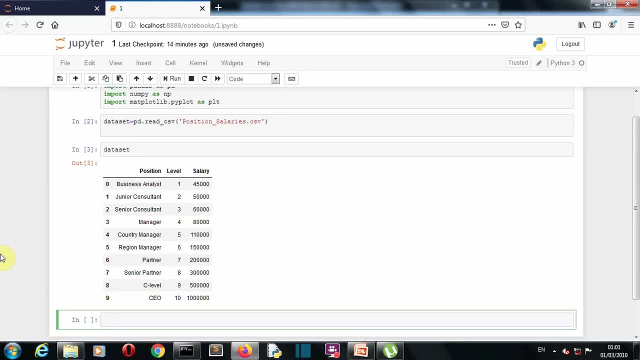 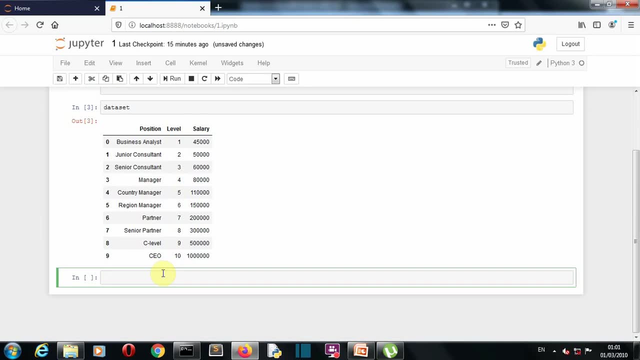 download this then. then go to the link in the description and you can find this data set, as well as this notebook, there. okay, so so now let's extract our dependent and independent data. the salary column is our dependent data and this level is our independent data. okay, 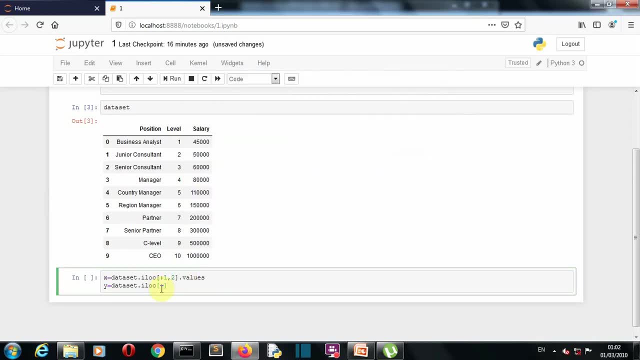 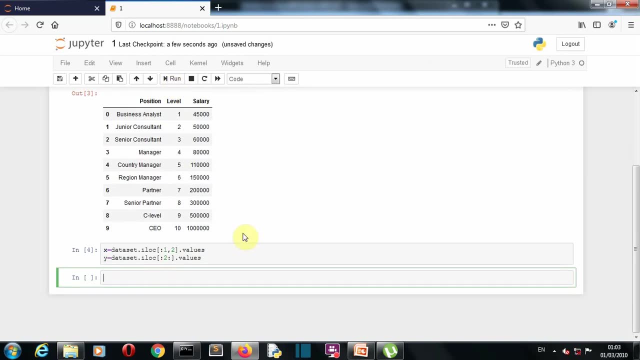 so now there is an extra step added for support vector regression, that is, feature scaling. now, if you don't know what feature scaling is, i have created a dedicated video for that. but to explain in short, feature scaling means making all the numeric data uniform, because there you can see. 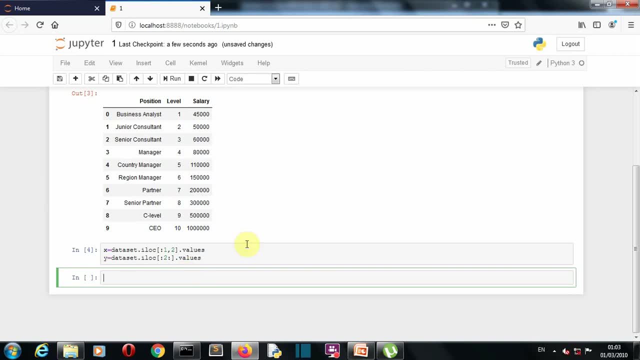 that the salary data is being used for the salary column and the value of the salary column is being is having high numeric value, whereas this level is is very small as compared to salary. so to balance them, we do feature scaling and in our previous models, like multilinear regression and 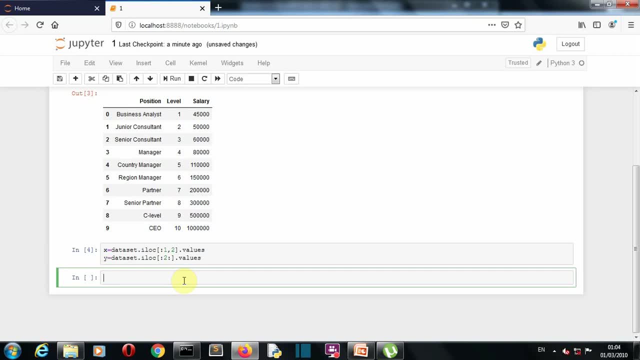 polynomial regression. it was already present in our package, but this svr is rarely used, so we have to do feature scaling here. and i have one announcement for you also, which i'll give after this video. so wait till the last of this video, because this is a very good announcement for you all, okay. 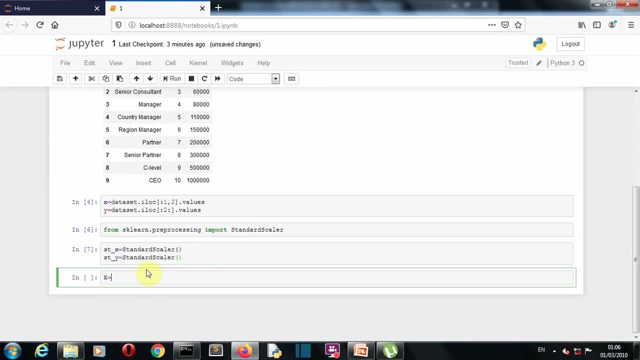 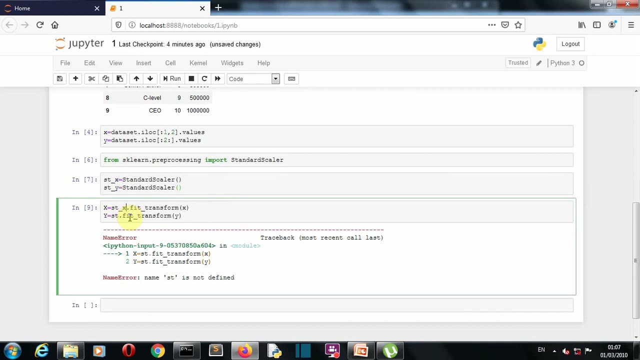 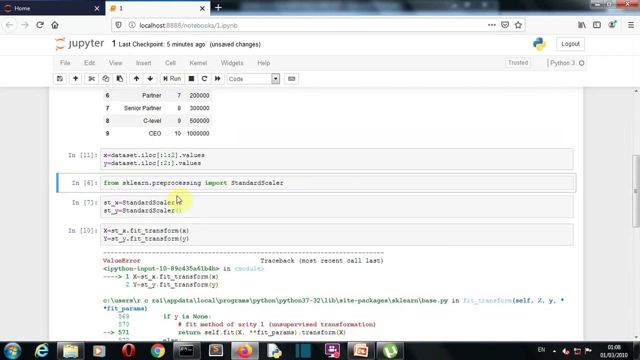 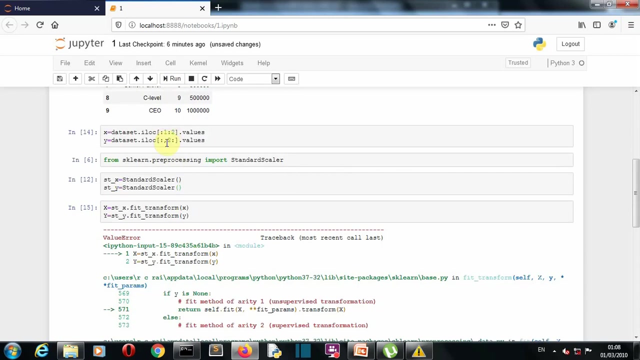 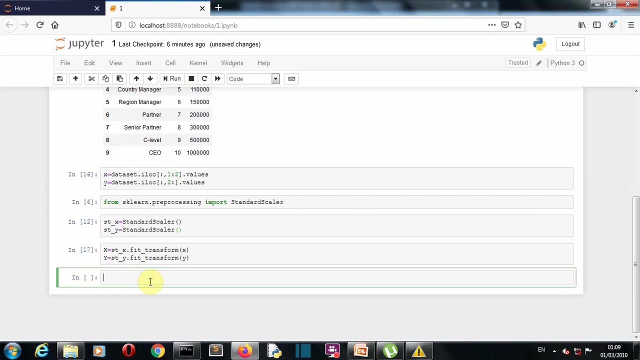 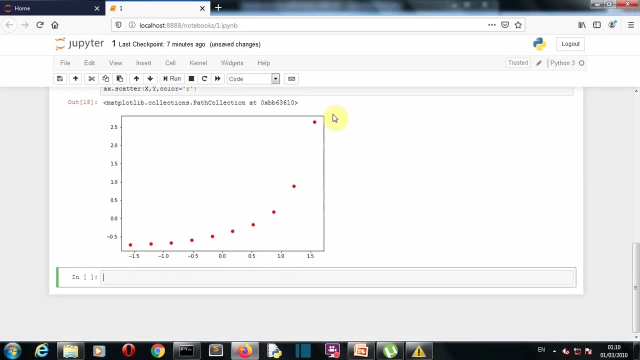 so let's go ahead and start the video. Okay, so now we are done with the feature scaling. Now let's plot our data points so that we can see that what is the trend. we will use matplotlib here, Okay. so there, you can see that our data set is following a polynomial pattern. 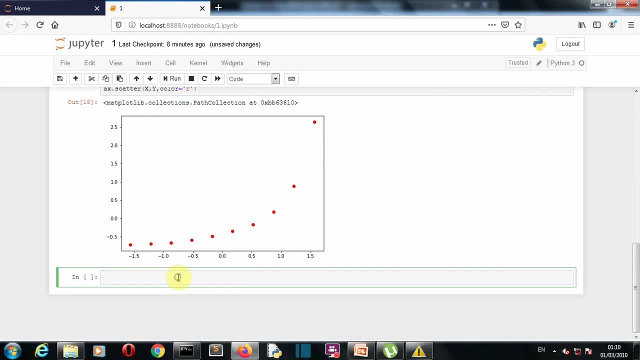 Okay, so now let's import our SVR package so that we can do our prediction. Okay, so now let's create our regressor object, so regressor is equal to capital SVR. make sure that this SVR is capital and then we'll decide that. what is the kernel? 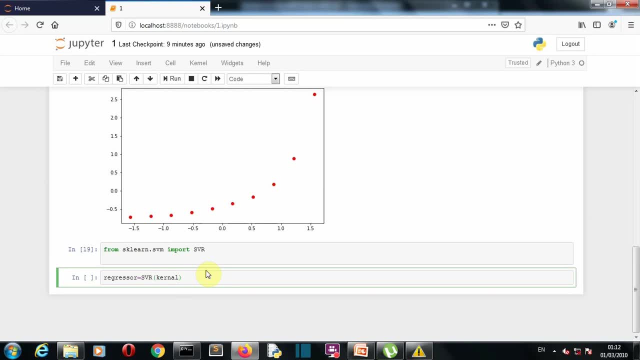 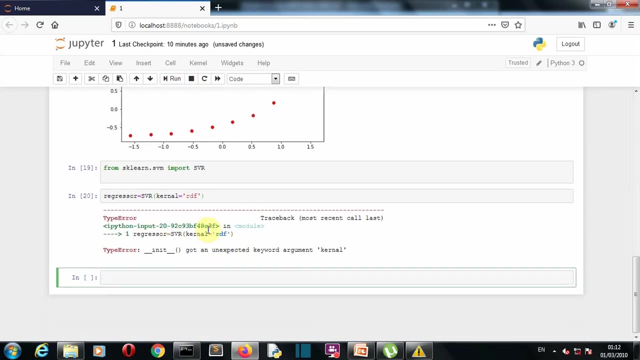 Now, kernel is the method or the model used, So by default it is RDF. you can use polynomial linear, any method that you want to use, but we are going to stick to our default one. So RDF It should be kernel, not kernel. Okay, now let's apply our regressor model to our X and Y data. 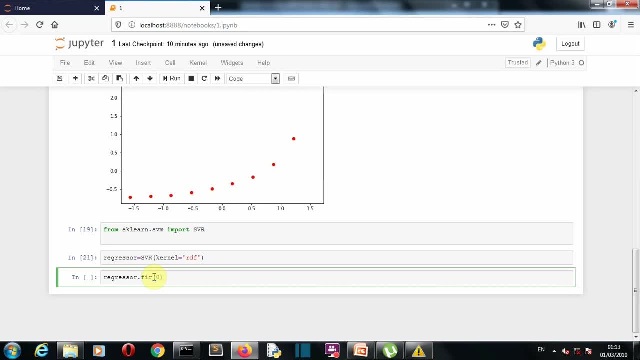 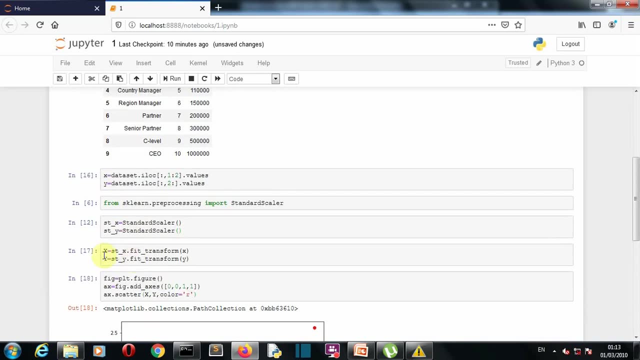 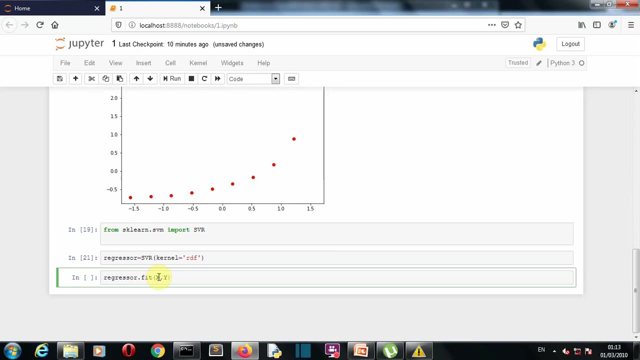 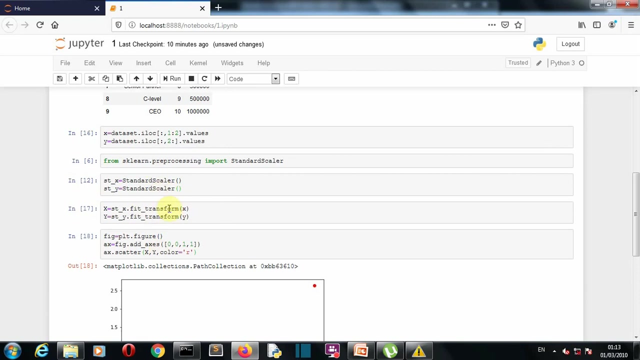 Okay, so we'll fit to. this should be fit here, fit to our capital X and Y, on which we have done our standard scaling. Okay, so I insist you to watch our video, Okay. Okay, feature scaling video first, because Without that you won't be able to understand that. why are we doing feature scaling here? Okay, 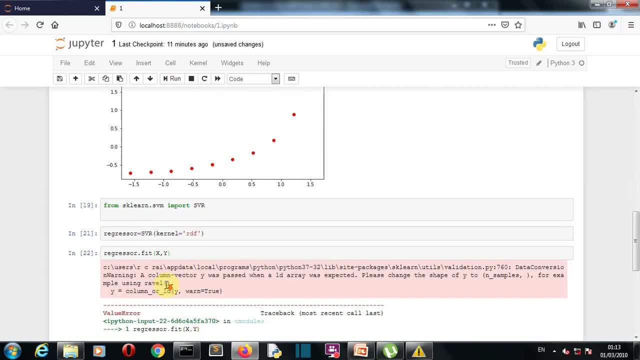 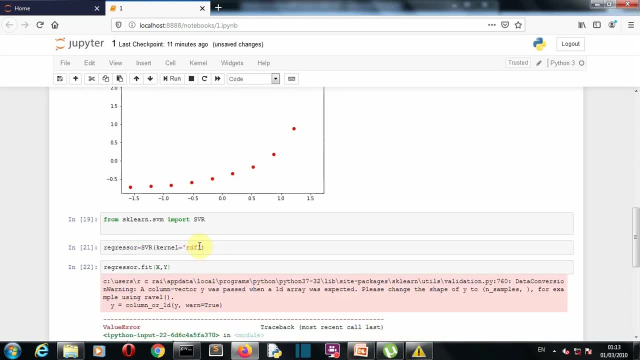 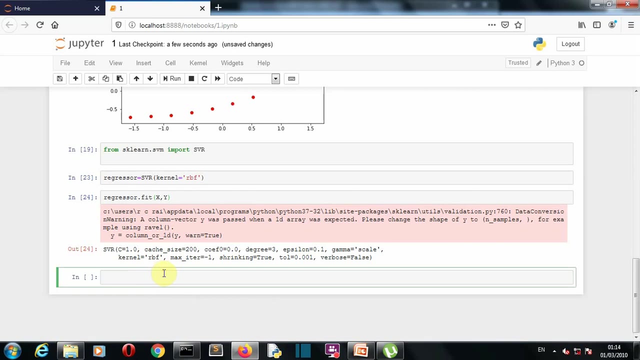 so Let me fit this. Okay, so we are getting a more warning. rdf is not defined, because this should be rbf. I'm sorry, Should be rbf. Okay, so we are getting a warning, but we are gonna Ignore that and our model is chained. 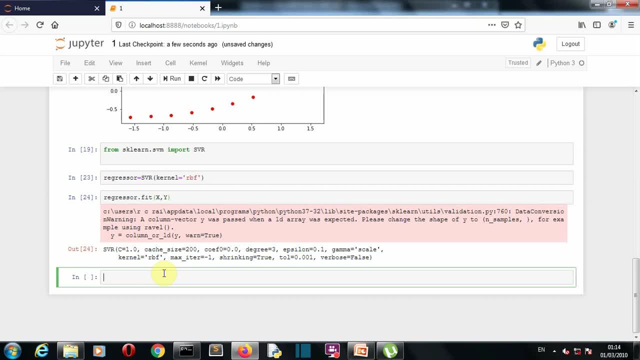 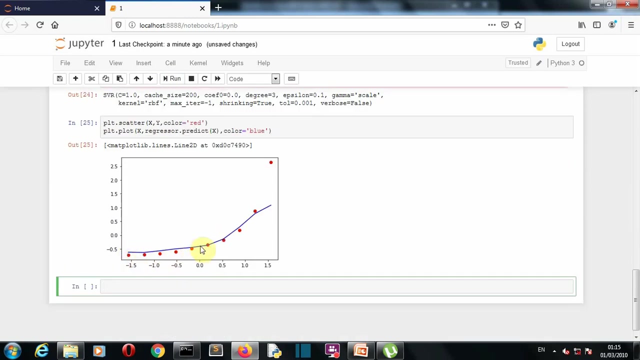 So let's plot our models To see that. what is the accuracy? Okay, Okay, so now let's run this and there you can see that our blue line is Prediction line and the red are our data points, so it is able to satisfy all the points and 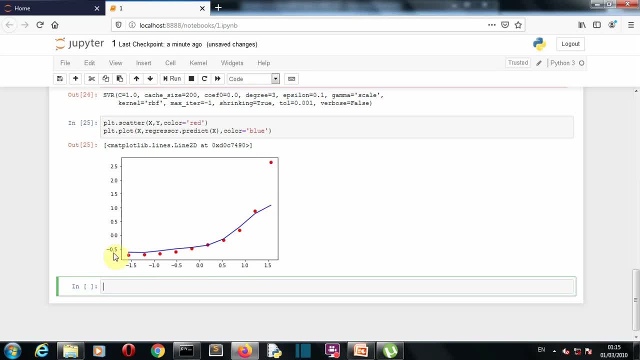 now this data point is not considered because our model is considering this data point to be as outlier. okay, to Avoid overfitting. So this is it. This was a short video in which I have explained you that what is svr and we have seen how. 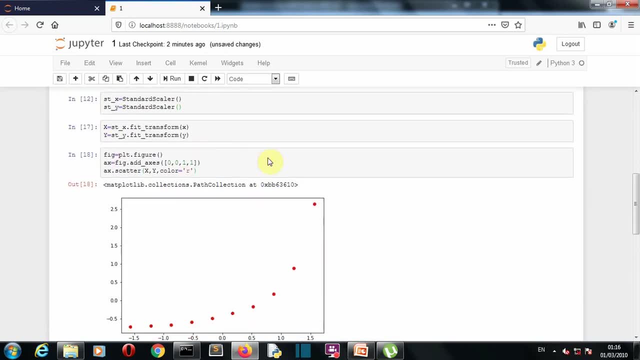 svr works on actual data set. now let's come to the Announcement. so the announcement is that if you are interested in social media marketing Or you want to know how I grow my social media- that is, my instagram page and my youtube channel- totally organically, without using any paid promotion or any of 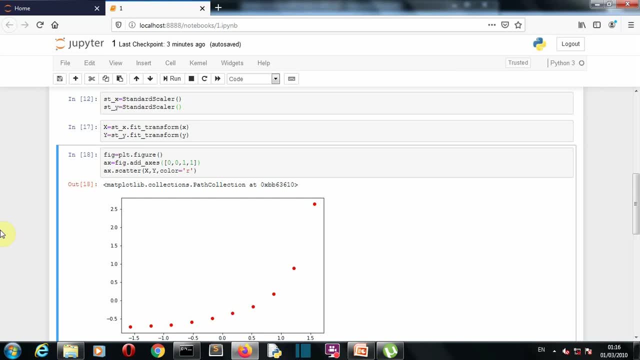 external support in just 3-4 months. then I have my channel Membership, on which i'll upload these type of videos, and not only that, I will regularly host members only live stream and members only chat, so you can join that, but This membership won't affect my regular videos.